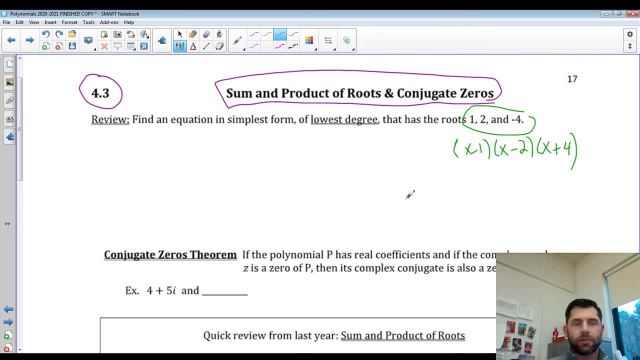 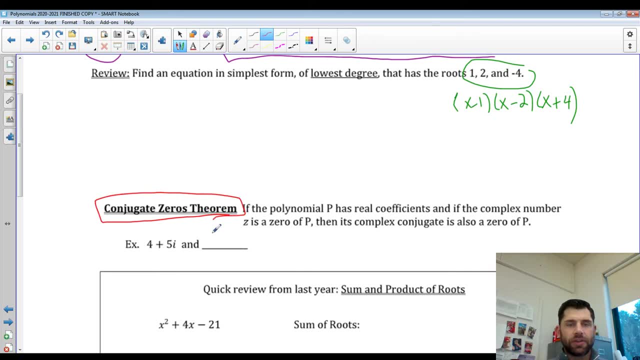 And we can multiply those through if we wanted to and we can get our polynomial, So we're not going to bother with that. Here's our first idea: the conjugate zeros theorem. If polynomial P has a real coefficients and if the complex number z is a 0 of the polynomial, 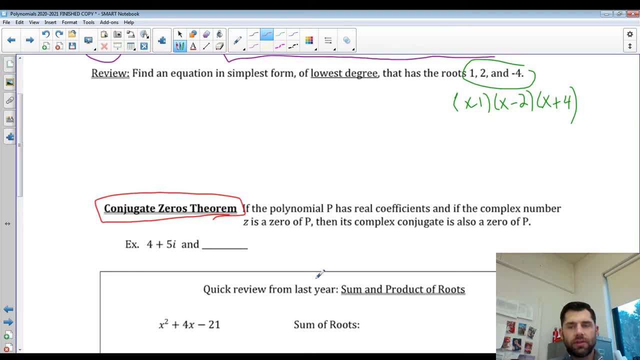 then its complex conjugate is also a 0 of the polynomial. So what that tells us, if you think about, if you were to solve an equation using the quadrilateral radic formula or completing the square at the very end, you would have something like this: 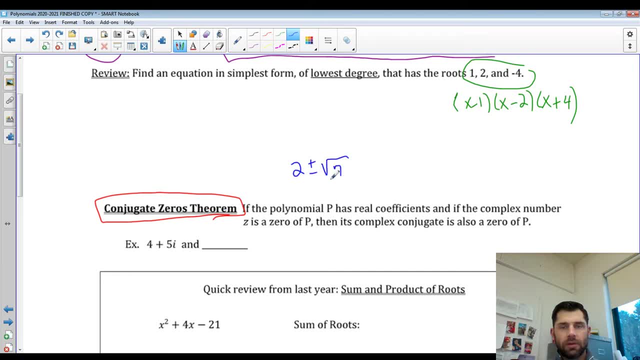 2 plus or minus, and then this could be anything. Let's say it's radical 7 over 4.. This plus or minus, it's always in the formula right. It never goes away. So unless this radical 7 part, unless this is like a perfect square. so if that was 9,. 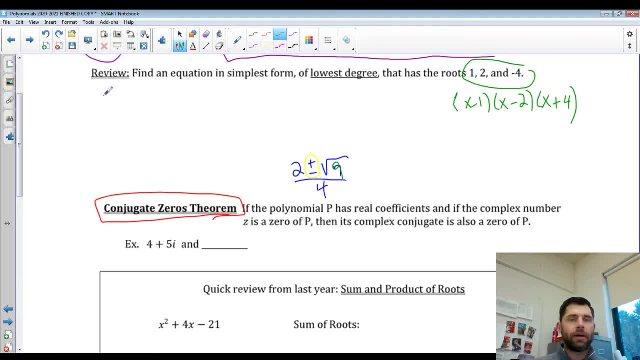 it would be 2 plus 3 divided by 4, and 2 minus 3 divided by 4, and that's your answer. But if it's a square root, you know an irrational number or an imaginary number. let's say it was like i radical 7,. 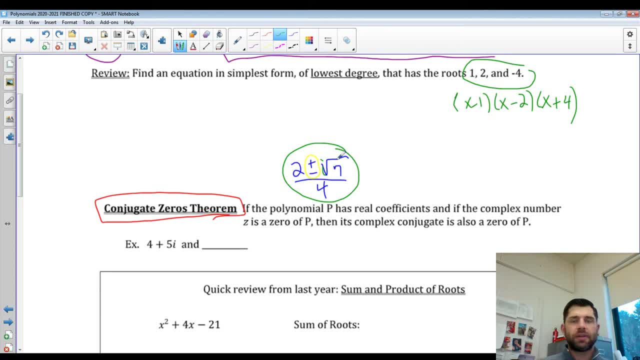 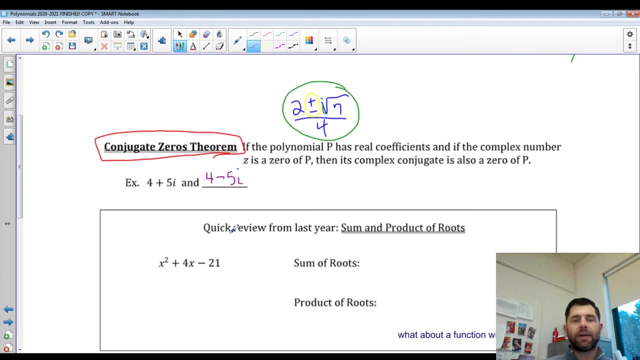 these complex numbers have to come in a plus and a minus pair. It has to. That's the only way that formula works. So, for example, if 4 plus 5i was a root, that means absolutely without a doubt, 4 minus 5i has to be a root. It has to work that way. 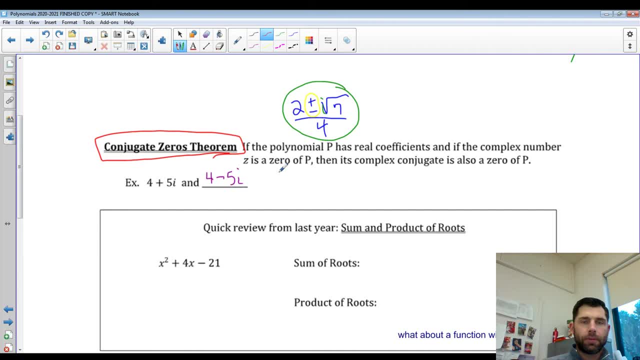 So just a little bit of foreshadowing. Let's say, I now wanted to turn 4 plus 5i and 4 minus 5i into factors. So just like you know, just like, let's say, x equals 4 was a root. 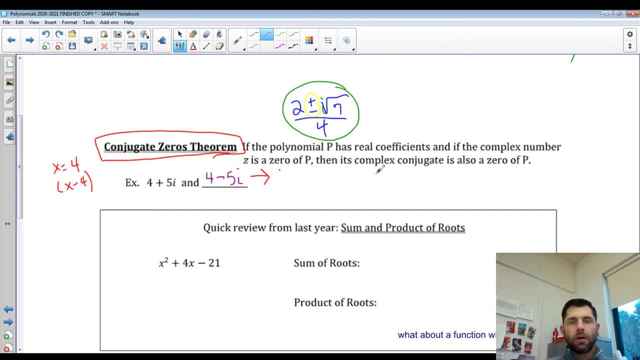 x minus 4 would have to be the factor. So if 4 plus 5i is the root, then x minus 4 plus 5i is the factor, And if 4 minus 5i is the root, then x minus. 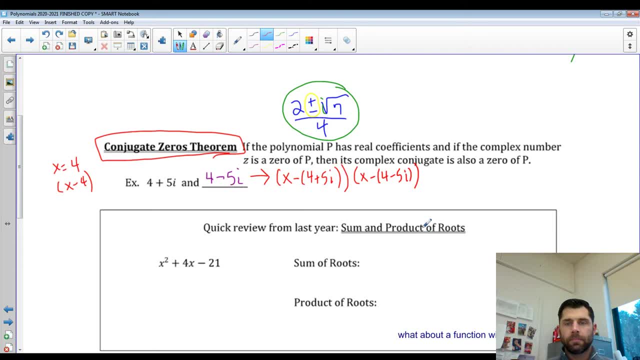 4 minus 5i is the factor, And then I could distribute that negative through and the factors would be a little bit nicer- Not really nice, but a little bit nicer. They would look like this: x minus 4 plus 5i. 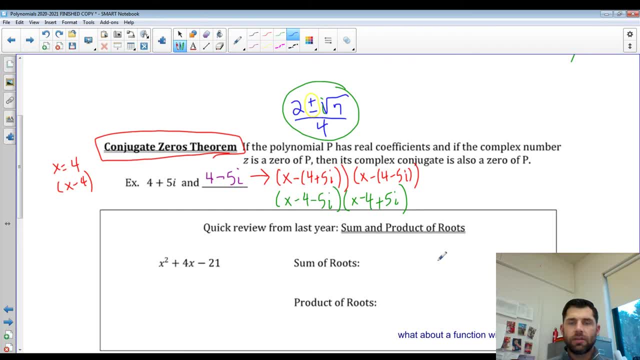 So here's what we're going to do today. We're going to learn a little shortcut here. If I wanted you to turn this into a polynomial, so with real coefficients to get rid of those i's, we could multiply that through and the i's would cancel each other out, basically. 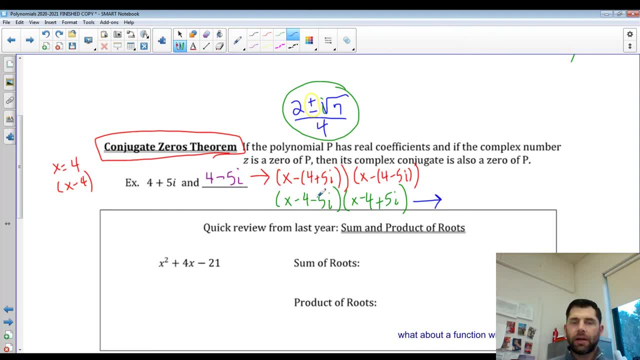 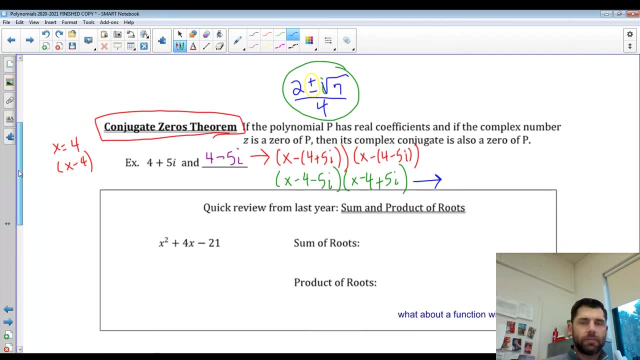 They would go away. But we'd have to multiply a trinomial by a trinomial and that would just become kind of a mess. So I'm going to show you a little shortcut, And this may be something you've seen last year, maybe not. 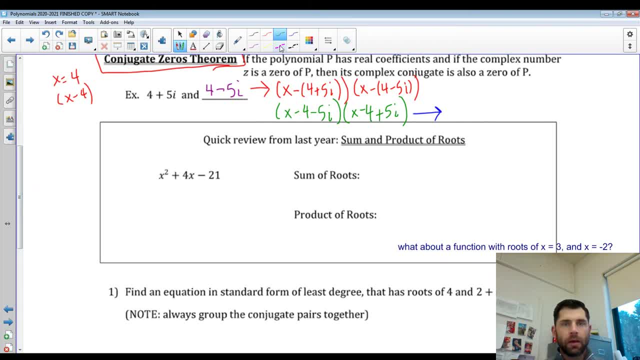 The sum and the product of the roots. Sum and product of the roots. So let's say I'm going to put an equal zero here. I want you to find the zeros or the roots or the solutions of this polynomial. So nothing to it. 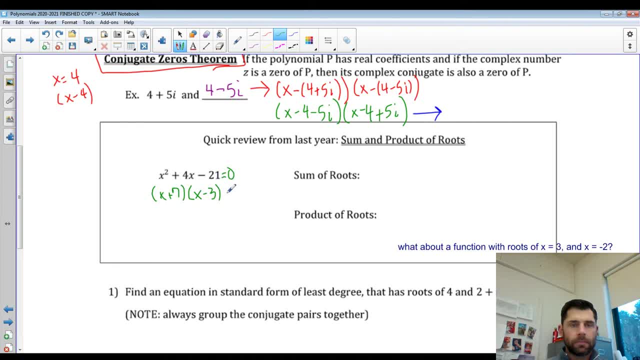 We factor da da da, We have x equals negative seven and x equals three. So what your algebra one teacher probably told you back in the day was, they said, once you get the factors you can just change the signs. So that was like a little shortcut that you learned. 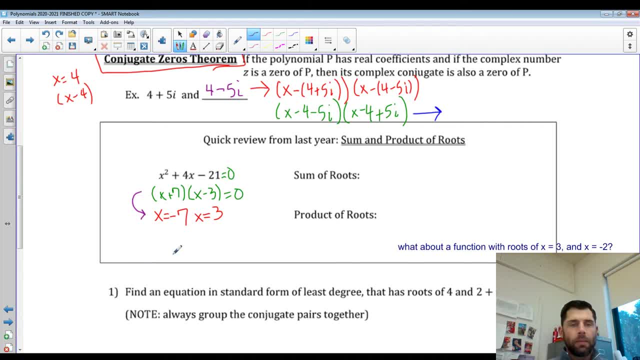 You probably know, well you know why that is the way it is now. But here's what's interesting about that. So if I take my two roots- the negative seven and the three, and I add them together, if I find the sum, 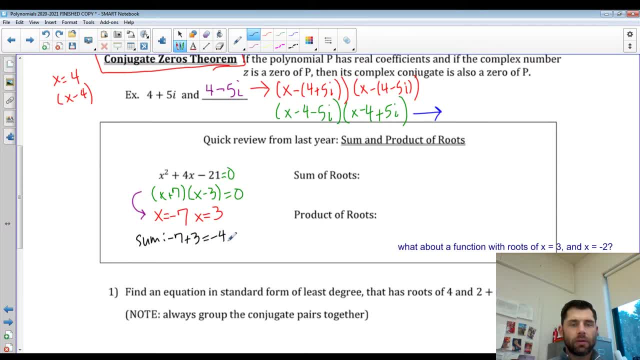 negative seven plus three is obviously negative four And I'm going to write it as negative four over one. If you look at how this relates to your original equation, the sum of the roots that negative four over one is the B value, just with an opposite sign. 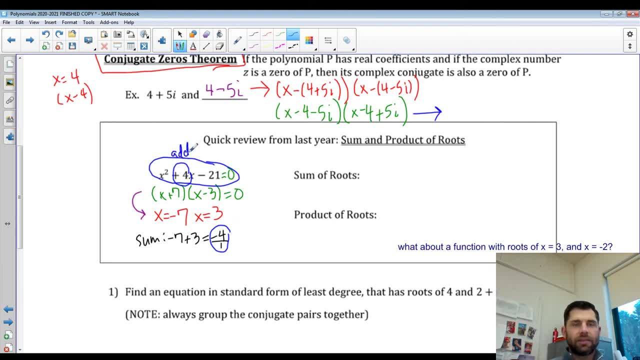 So if you think about back in algebra one again, you would think to add to a positive four and multiply to a negative 21. So if we're looking for numbers that add to the positive four, but then we chicken out, switch the signs when we're finding the solutions, it makes sense that if I add my solutions together 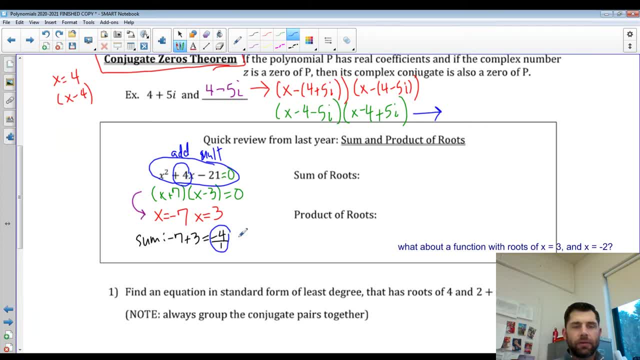 it's going to be the opposite sign of my B value. So this formula, this sum of the roots, if I add my roots together, it always gives me the B value, just negated over whatever the A value is. In this problem, the A value is just one. So the sum of the roots, if I add my roots together. 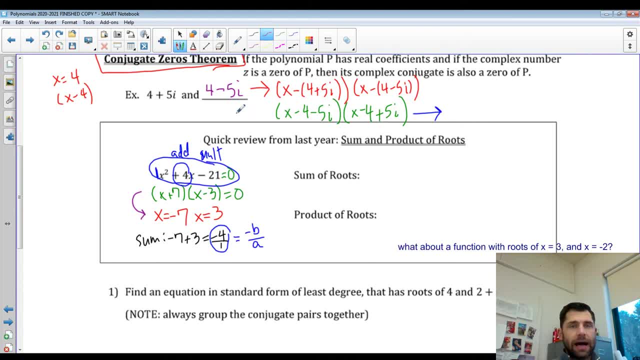 it tells me exactly what the B value is, just the opposite sign. And the product of the roots is even easier. If I take negative seven times three, that equals negative 21 over one And you can see right there: negative 21 is my C value. 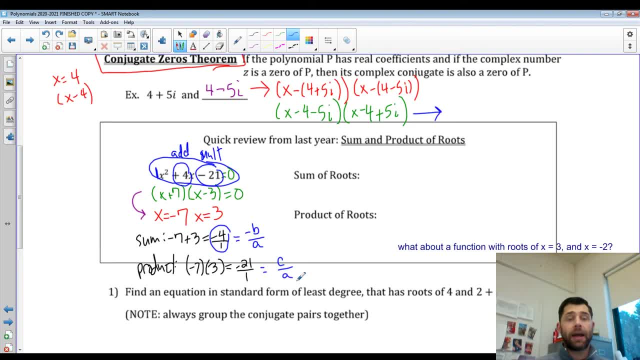 So the sum of the roots. if I know the roots of a function and I add them together, that tells me what the B value is. And if I multiply the roots together, if I find the product, that tells me what my C value is. 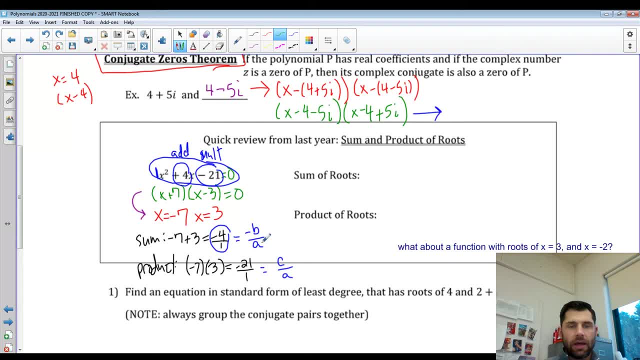 And then if they have a denominator, if they have a common A value here in the denominator, that tells you what the A value is, All right. So formula: the sum of the roots is negative, B over A, And the product of the roots is C over A. 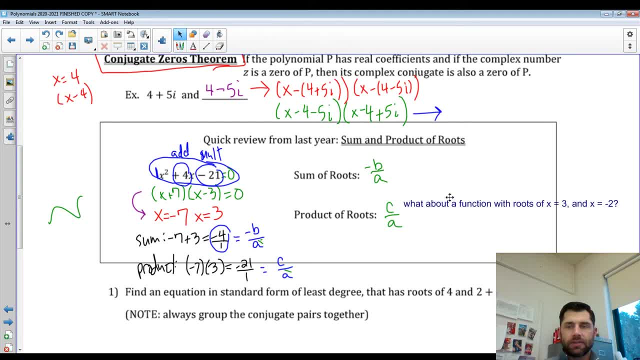 So once we do a couple of these, that will make a lot more sense. All right, So what about a function with roots of three and negative two? This one, you don't really need to do the sum and product of the roots. What we could do is just you don't have to write this. 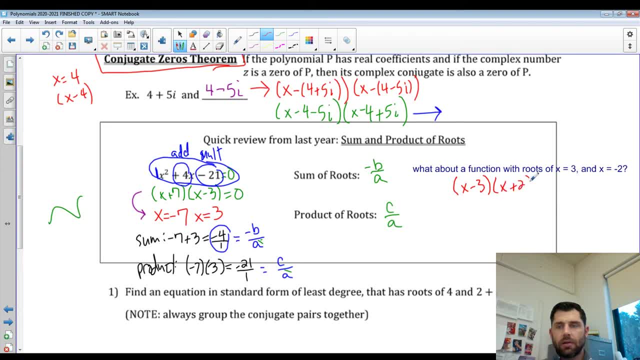 but we could just turn these roots into factors. right there We can multiply it. We would get X squared minus X minus six, So that one. you wouldn't need to do that formula. It's really easy to multiply. But just to show you how to do it, I'm going to show you how to do it. I'm going. 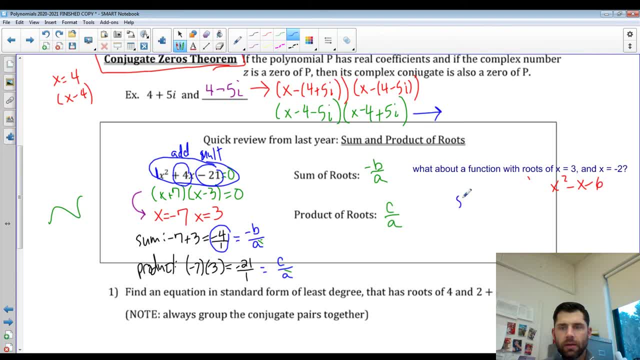 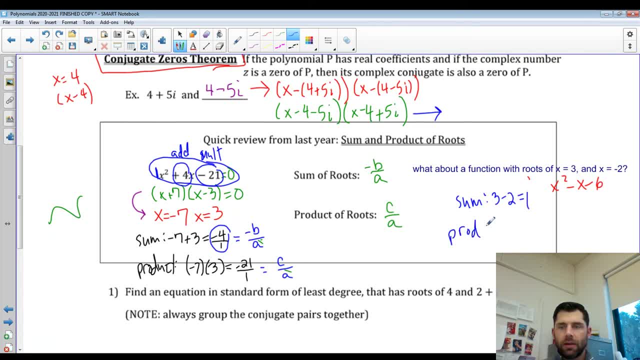 The product of these roots three times negative. two is negative six. So you can see, I can take those values. The B value would be negative, one which it is, And the C value would be negative six which it is. So I'm going to show you how to do it. I'm going to show you how to do it. 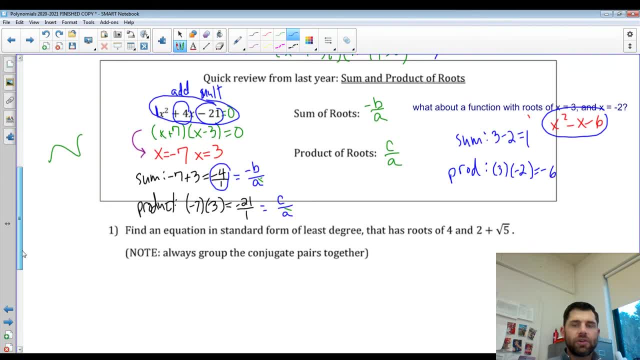 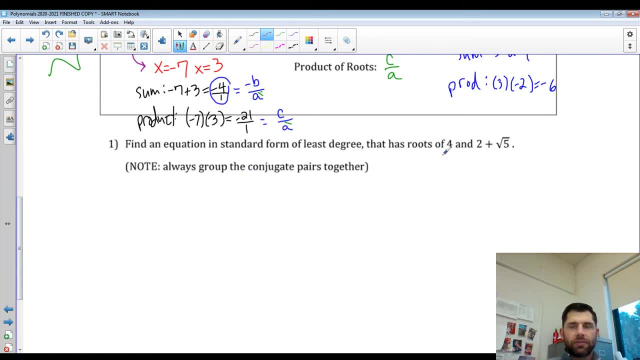 So it's a little bit of a nice streamlined process when we're looking at a question like this. So find an equation in standard form of least degree that has roots of four and two plus radical five. So first thing, here's my roots: X equals four, X equals two plus radical five. 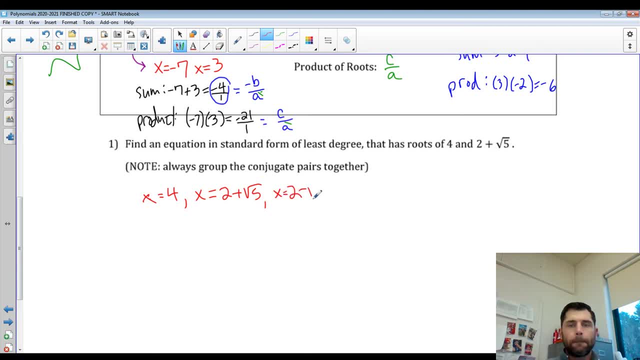 And don't forget the conjugate pair. X equals two minus radical five. So what we could do to find this polynomial, I could do X minus four. Careful here: X minus two minus radical five, So turning these roots into factors, And X minus two plus radical five, If you don't want to learn this new process. 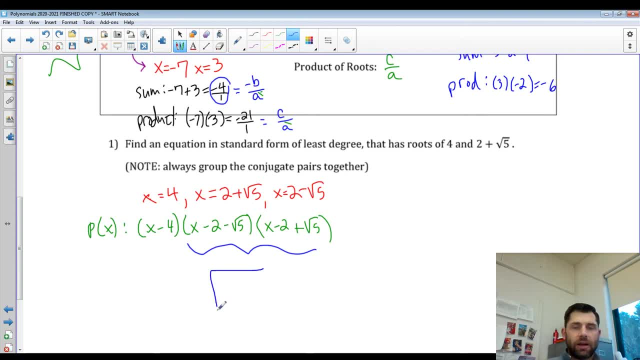 you could multiply those together. You could do a trinomial times, a trinomial. like I said. You could go to your windows if you need to And you'd be here for a few minutes. It's not the worst thing in the world, but there's an easier. 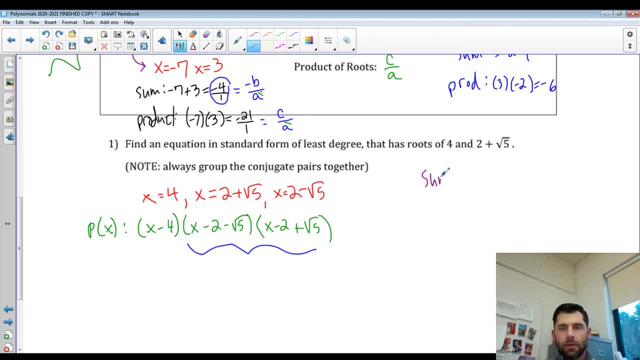 way We can use this sum and product of the roots process. So, looking at my roots, I have two plus radical five. I have two minus radical five, The sum of those roots, and this is why it works. This is why it's so nice with these irrational and complex roots: Two plus radical five. 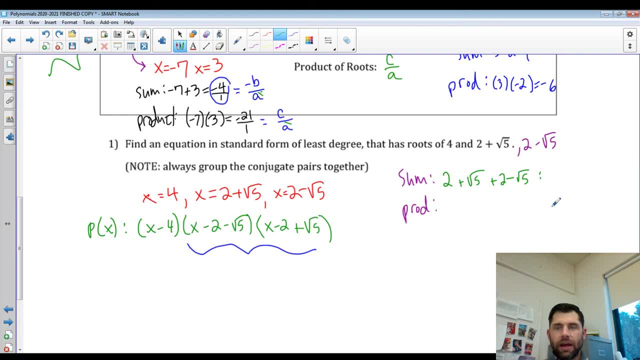 plus two minus radical five. Those radical fives go away. They add to a zero. So my sum is just four, My product: two plus radical five. two minus radical five. That's great. We already see the pattern. This is a difference of two perfect squares really. So we have four minus two radical five. 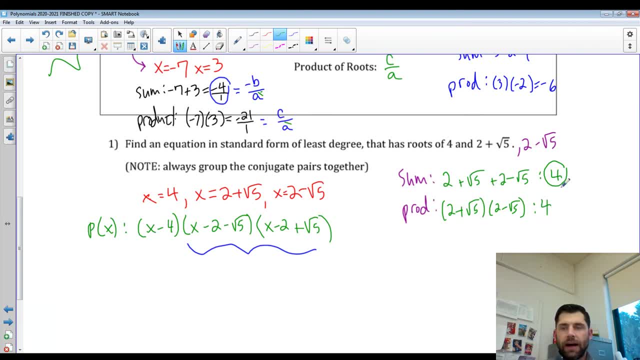 plus two radical five. So those radical fives go away again and we're just left with four minus five, which is negative one. There's the product of the roots. So we're done. That's my answer I have. that should be an equal sign. I have. p of x equals x minus four. 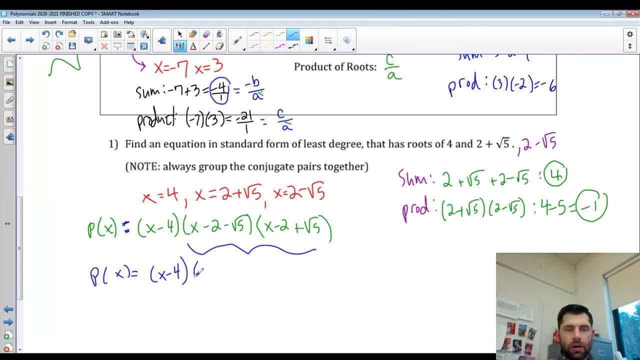 And then I can turn these two complex roots into a quadratic really quickly. So it's x squared, My sum is four. So in the formula my b value is negative four And then my product is negative one. So that's all there is to it. 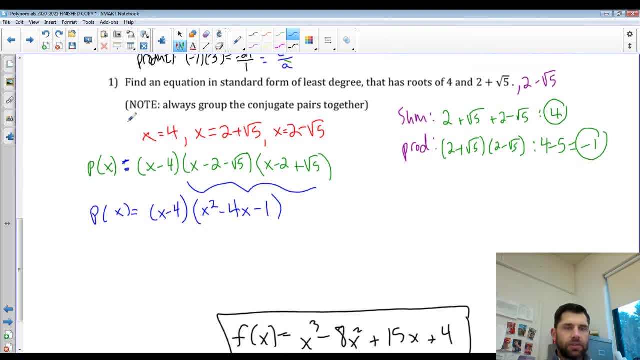 Now I didn't give you a point to go through, I didn't tell you like specifically what to do, So we're just going to leave it there. We can multiply it through. I did that for you because I know you guys can handle that. 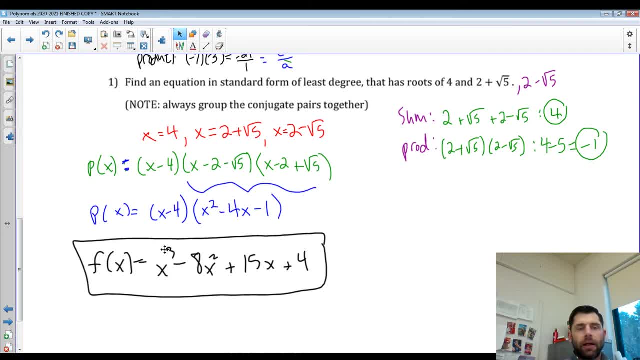 So there's how we would find our polynomial, And I just changed it from a p to an f, whatever You guys know what I mean. So it just streams out. It streamlines the process. So let me go to the next page. 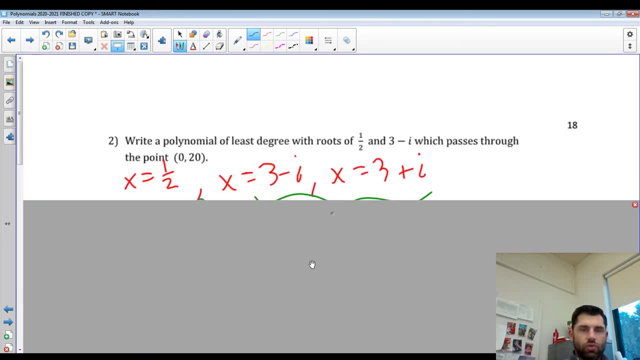 Let's see what I want us to do here. Why don't you guys, why don't you guys do number two? I'll pause and let you work on it. I have my work done, So just to see how you did. If you are lost, you can just wait for me to unpause it. 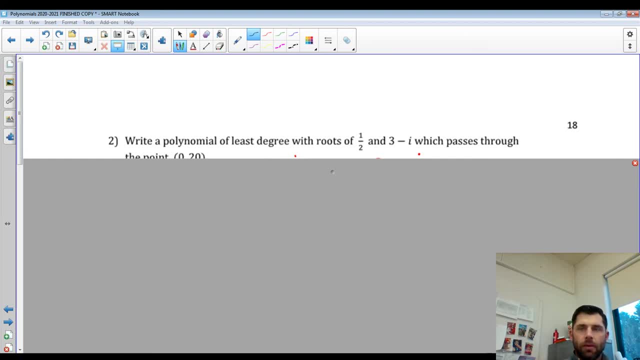 And then we will go through it together. So pause now, Try it out. We'll talk again in a minute, Okay, So hopefully you paused and gave it a shot. So there's my roots: x equals one half, x equals three minus i. 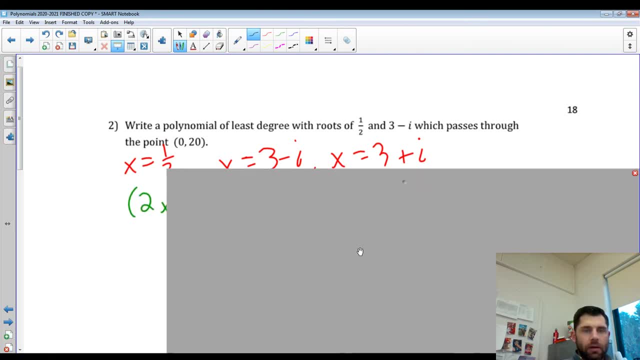 x equals three plus i. I mentioned this last time. It's a lot easier when we're doing our multiplication to turn that one half into a two x minus one. You don't have to, But it's nice to do it sometimes. Make your life a little easier. 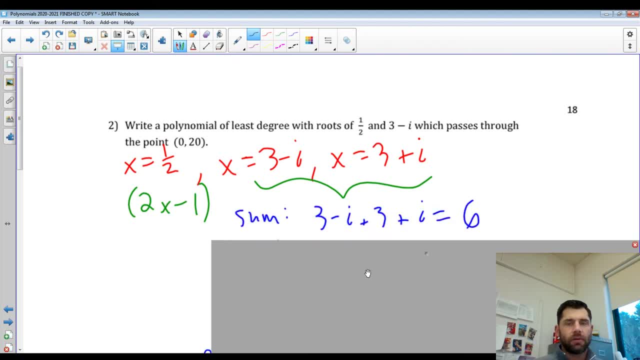 And then I would encourage you to get a little practice with this. So we do our sum of the roots, We do our product of the roots. Side note, just in case we didn't mention this in class. i squared, if you recall, is equal to negative one. 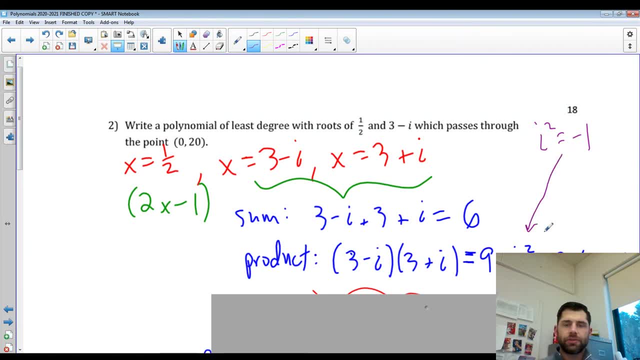 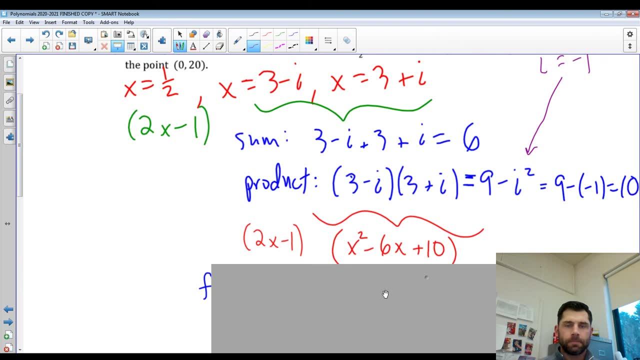 Alright, so that's what I did right here. Sum of the roots- Product of the roots. So my sum is six, My product is ten. And now we're set up. I still have my two x minus one. My sum is six. 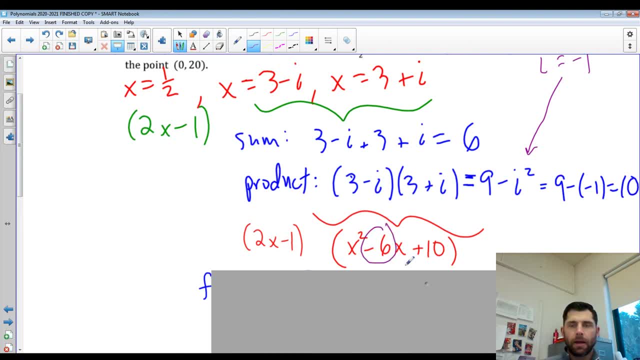 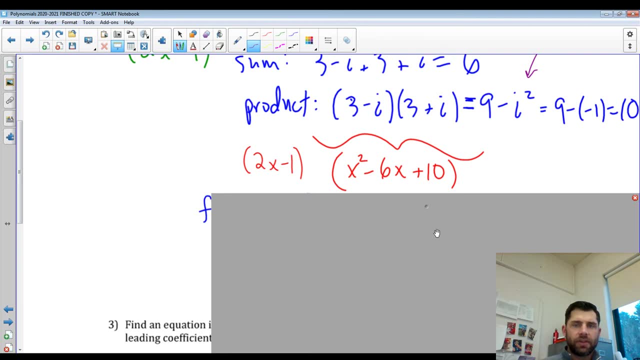 So it's a negative six in my quadratic And the product is ten, So it's just a ten in my quadratic. Okay, so pause if you need to look at this more closely. But I can distribute, Combine some like terms And then the one thing I did tell you for this: